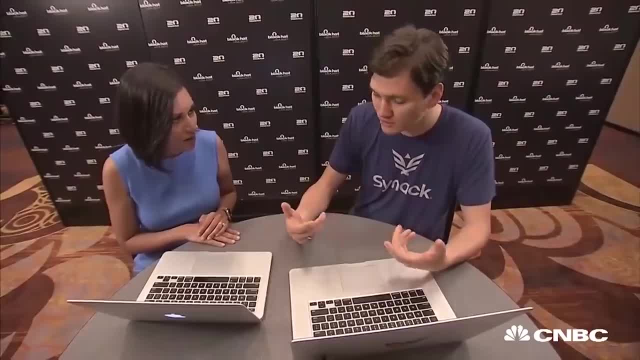 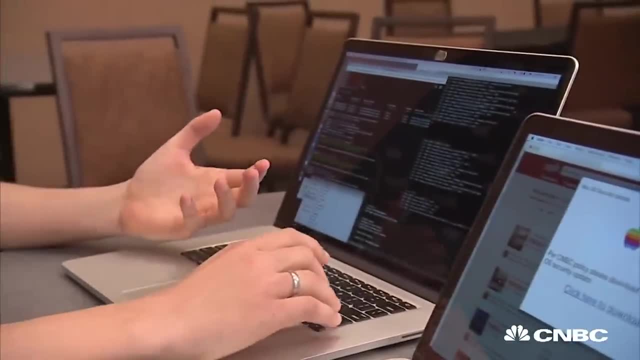 it recorded the picture, but you can actually record the video. You can also record sound if you wanted to. That's really disturbing. You can execute things on the behalf. So what I'm going to try to do is actually open the calculator application. Okay, Here we go. There's my 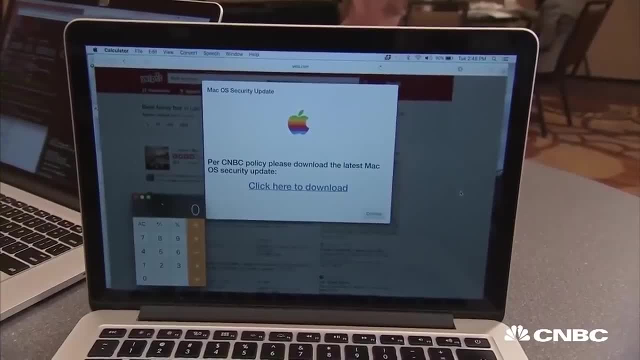 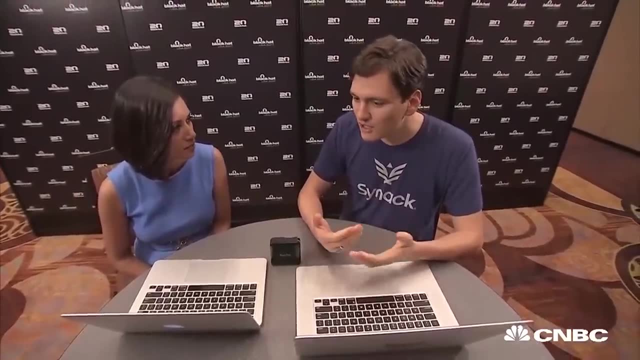 calculator just popped up, I can basically execute any types of commands I want on your behalf. So what can people do to protect themselves? You should sort of be on the lookout for anytime you sort of do an action and then the computer asks you to do something on your behalf. 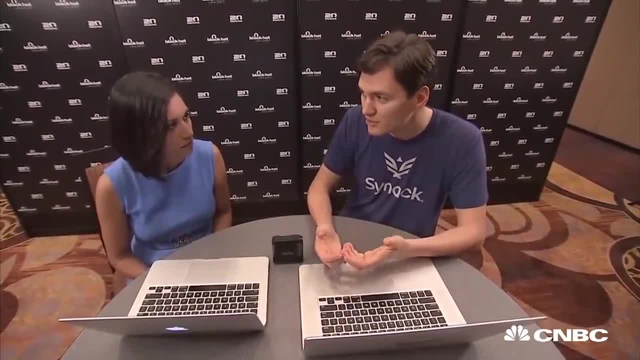 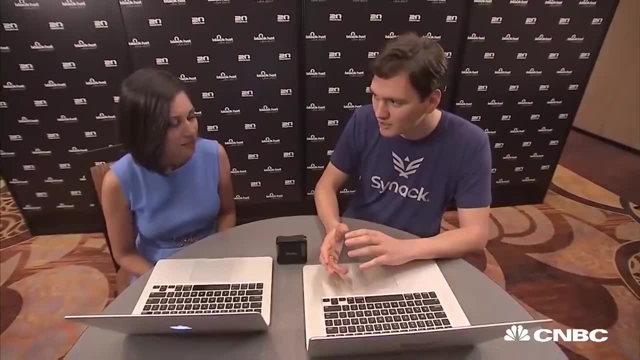 Like you know, you downloaded something and said, hey, please enter your password. You know, if you didn't expect that to happen, maybe you should kind of stand back a little bit and say: well, does it normally happen when I log into a Wi-Fi access point? 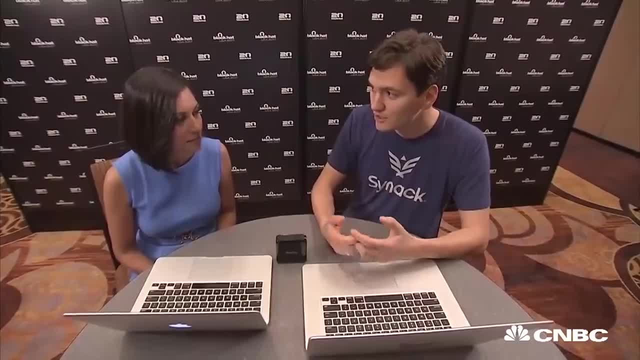 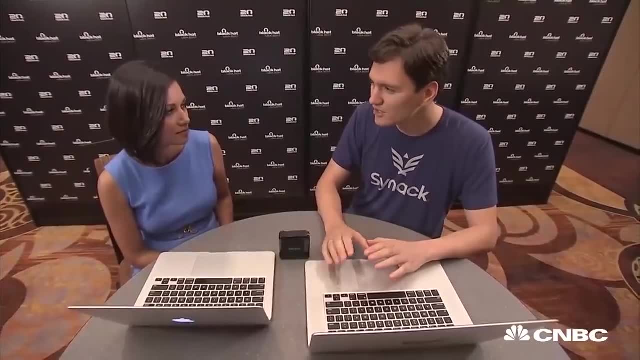 Or if you are logging into a network and you didn't expect to be redirected to an update page. you know, you should kind of stand back a little bit and say: actually I'm not going to download this until I go home and I can trust my Wi-Fi. Well, thank you so much. Great to see this.